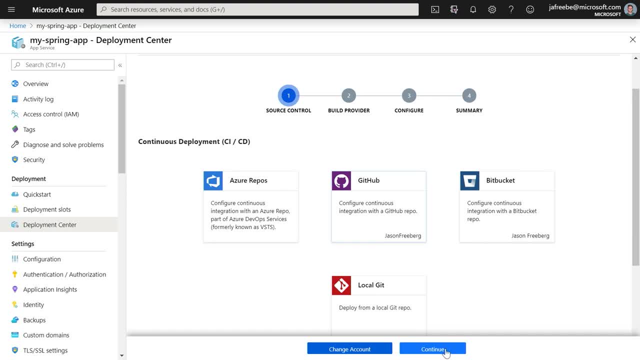 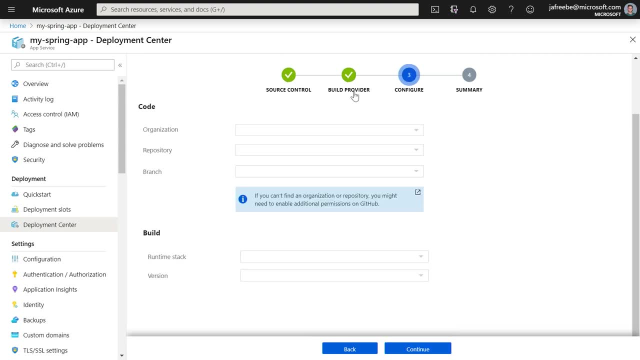 talking about GitHub Actions, So I'll jump into GitHub and hit continue. Now on this screen we have a new option for GitHub Actions, So I'll select that. And now on this next screen, I'm going to select my repository, So I'm going. 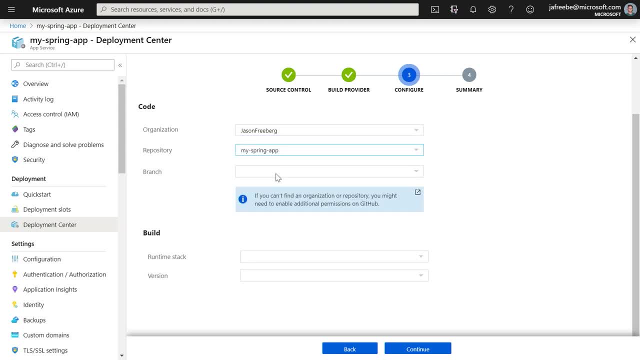 to select my username and then my spring application that I'm going to deploy. Here I'm going to deploy my master branch- It could be any branch, but I'll choose master- And then here I'm using Java 8.. And since I'm deploying a Spring Boot, 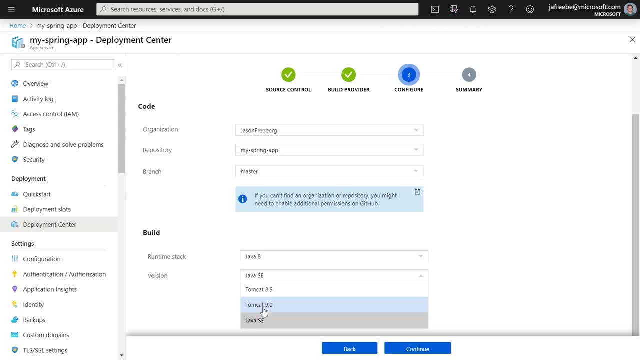 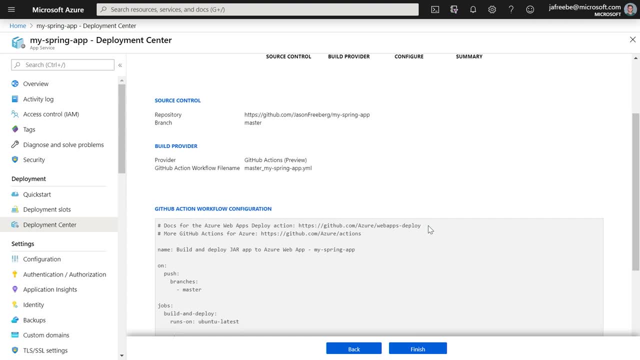 application, I'm going to choose Java SE. If I was deploying a Tomcat application, I could choose one of these Tomcat versions, And so now, on this last screen, we have a summary of my selections here so I can go back and edit, And at the 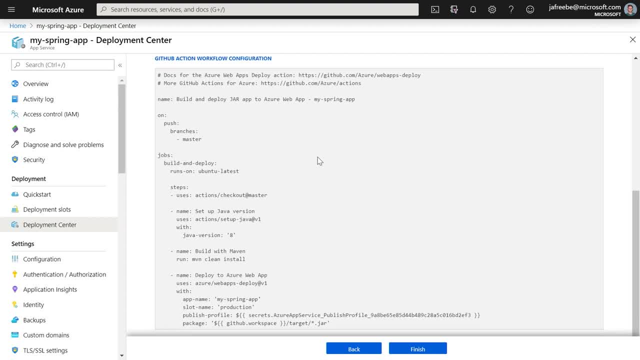 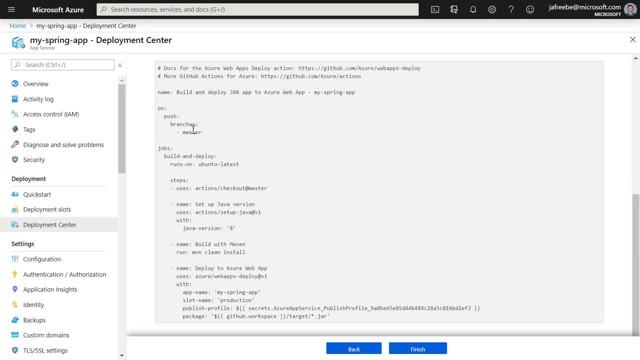 bottom we're looking at a preview of the workflow file that will be committed into my repository. So if we take a quick look here, this will run anytime that there's a push on the master branch. This will check out the master branch of my 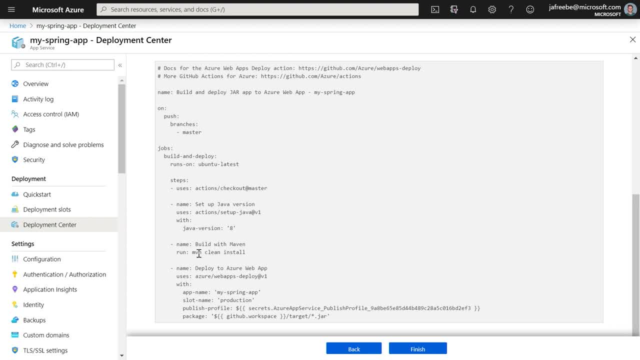 repo set up my Java version to Java 8.. It'll build my Spring app using Maven And then finally, using the deployment action, it will grab that jar file and then deploy it onto my web app. So when I click finish here, this will start the process to. 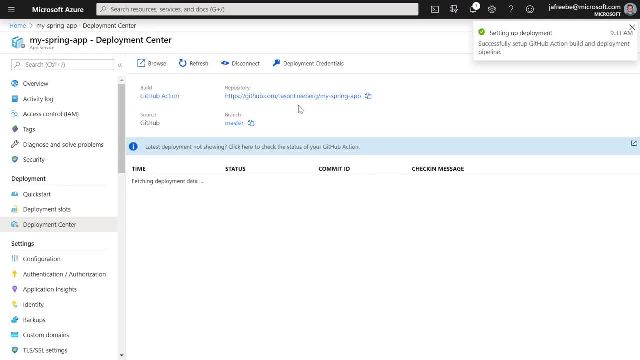 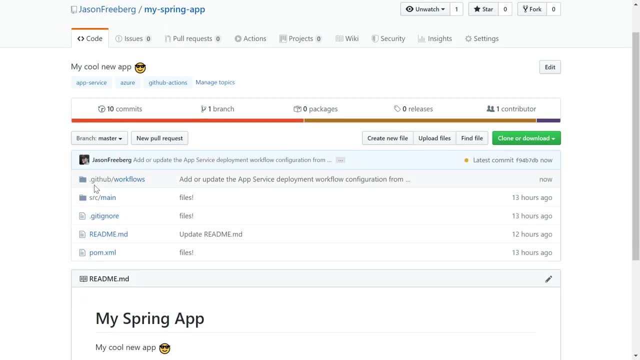 commit it into my repository And let's go ahead and jump into my repo using this link right here. So there's a new directory in my GitHub repo: github- slash workflows. So, as you might guess, this is where all of my 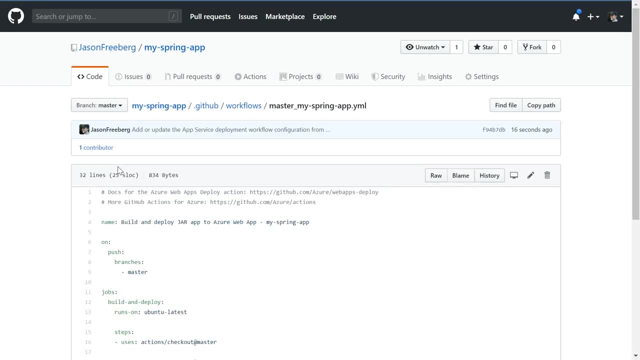 workflows would be. Right now I only have the one that was just added And if we take a look at the file, it matches the one that was shown in the preview just a minute ago. So what I'll do now is come up to the top toolbar here, select actions and this: 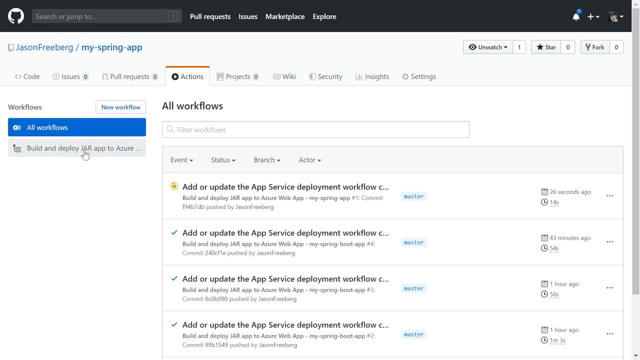 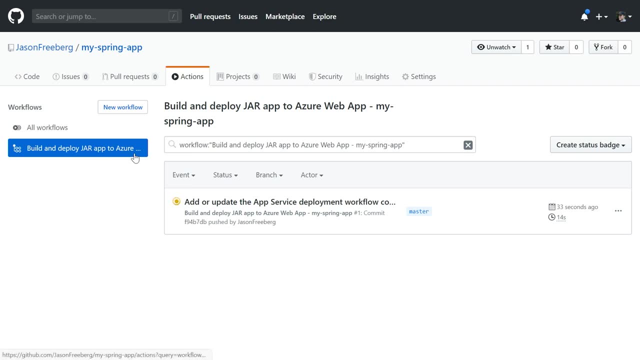 shows me all of my previous workflow runs and on the left-hand side it shows me all of my different workflow files. Now, in this case I only have the one, So I'll select this workflow file right here and we can see that that deployment action is.